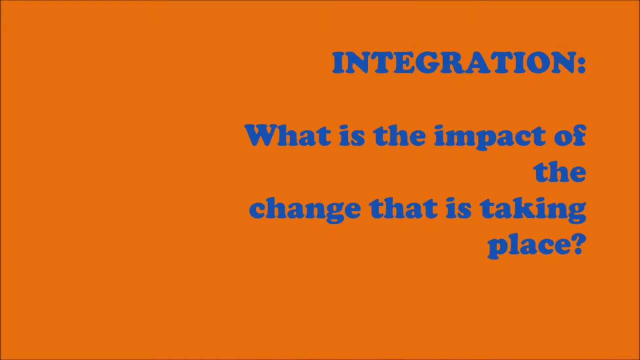 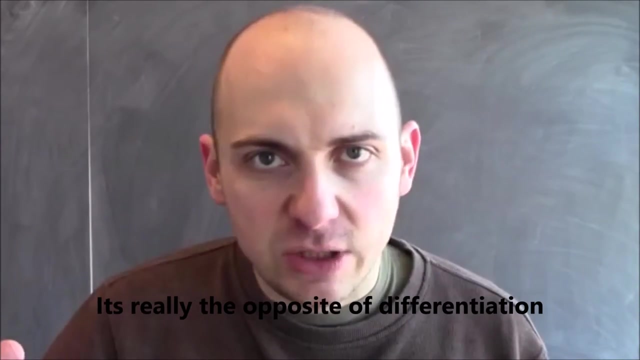 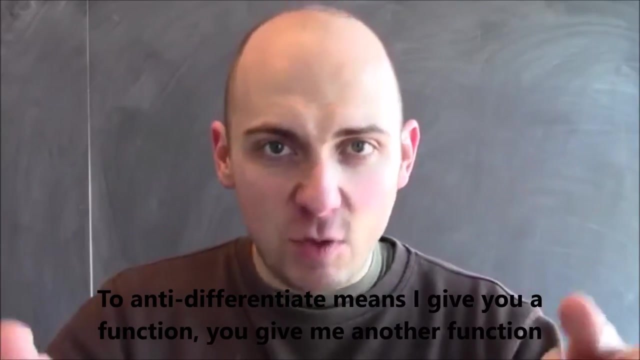 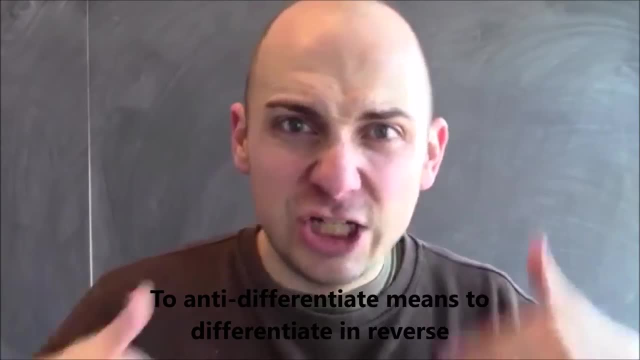 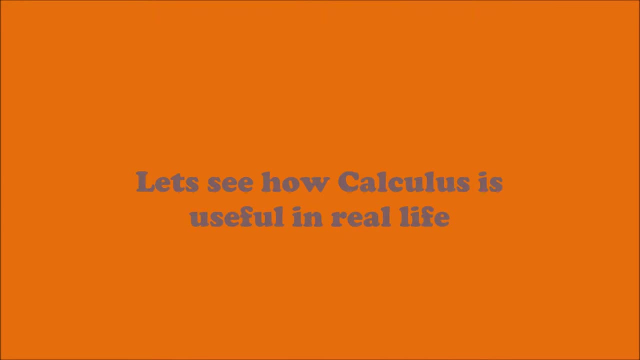 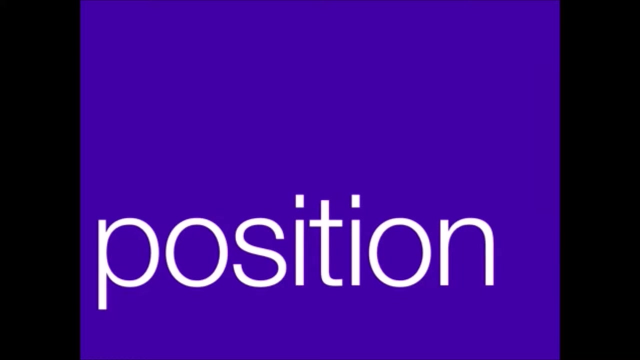 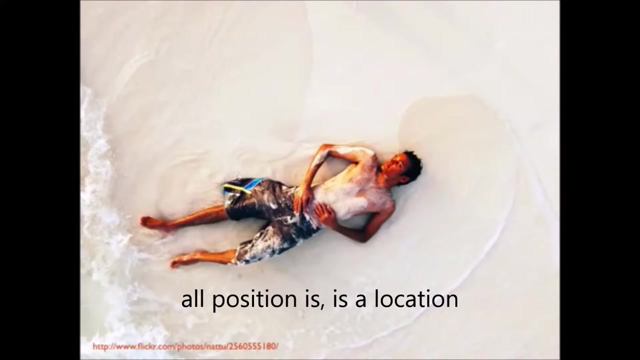 you right To anti-differentiate means to differentiate in reverse: right To start with a function and find a new function whose derivative is the given function. Position in the physics equation is labeled x and has units meters. All position is is a location, It's where something is in the world. It's x marks. 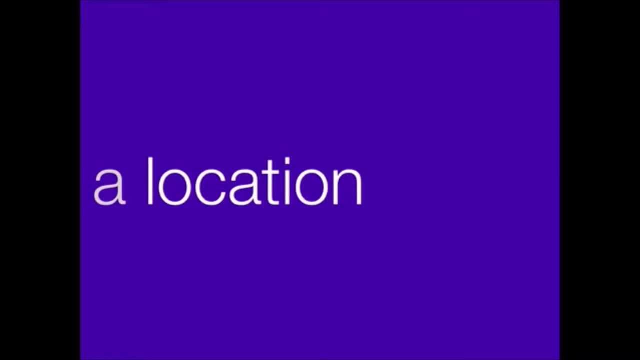 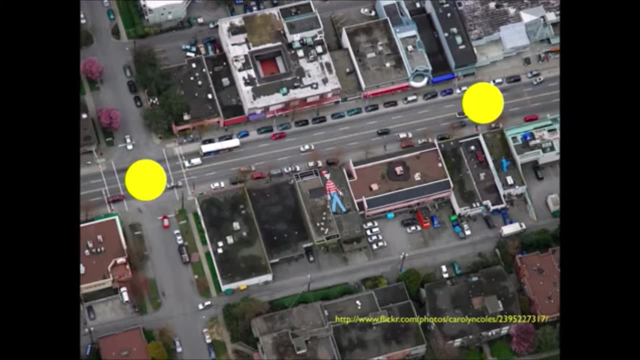 the spot Position is a location. A car starts here A couple seconds later it ends here. The first yellow dot is the initial position. The second dot is the final position. This change in position going from one location to the other is distance. 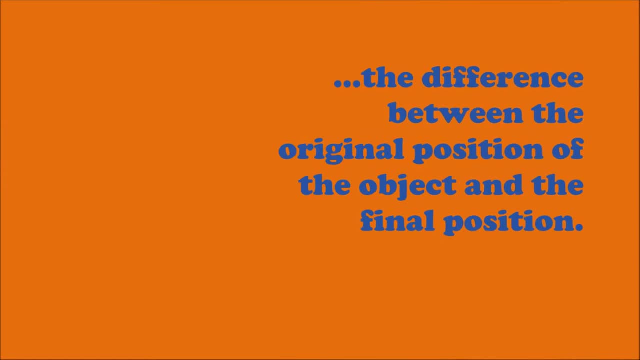 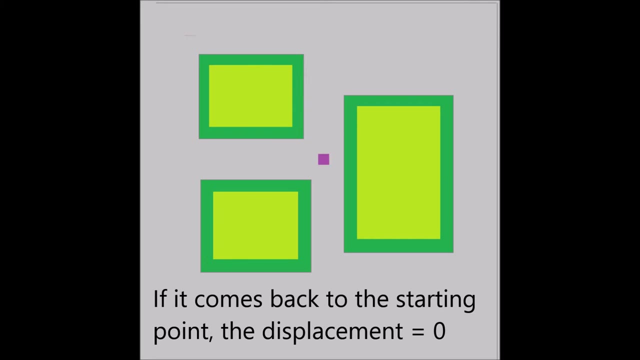 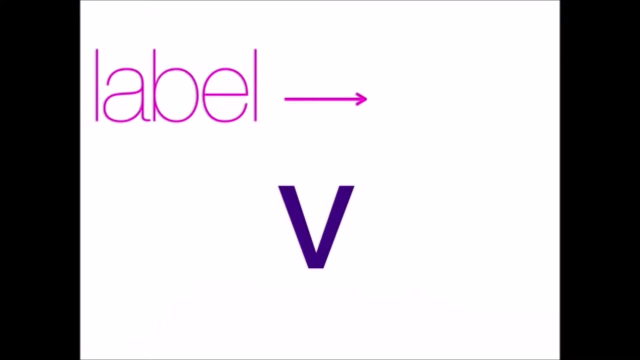 If the object moves, displacement is the difference between the original position of the object in the final position. So no matter how much distance an object covers, if it comes back to starting point, displacement equals zero Velocity. Velocity in a physics equation is labeled V and has units meters per second. All velocity is is. 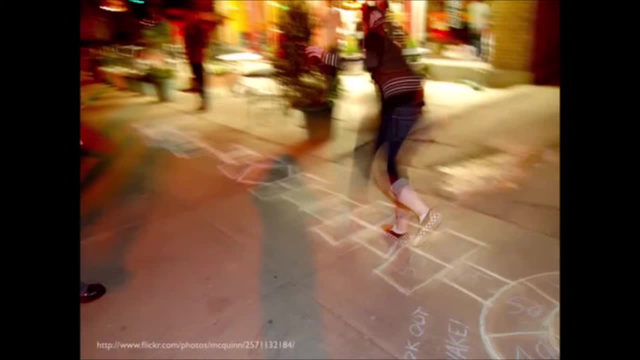 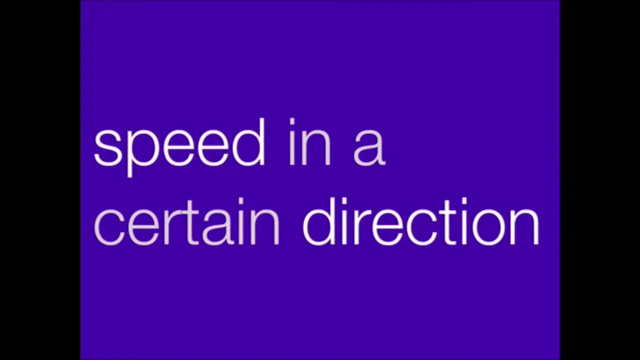 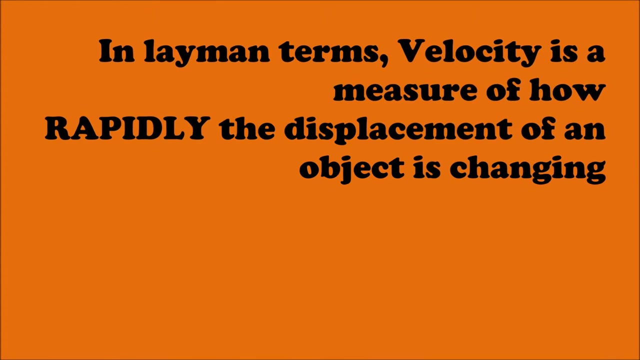 speed in some direction. It's how long it takes you to go from here to there. It's cruising in your car heading east. Velocity is speed in a certain direction. In layman terms, velocity is a measure of how rapidly the displacement of an object is changing. 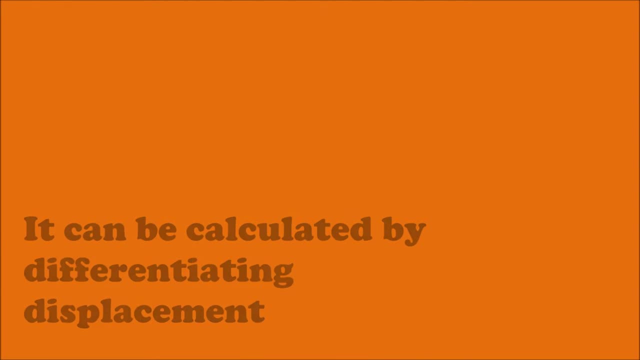 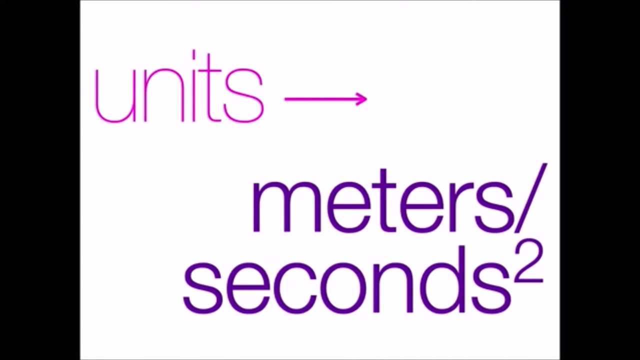 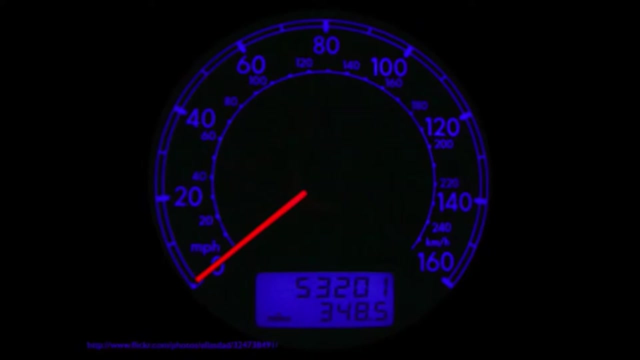 It can be calculated by differentiating displacement Acceleration. in a physics equation is labeled a and has units meters per second squared, and all acceleration is is the change in velocity per time. It's speeding up and it's slowing down. It's a Ferrari selling. 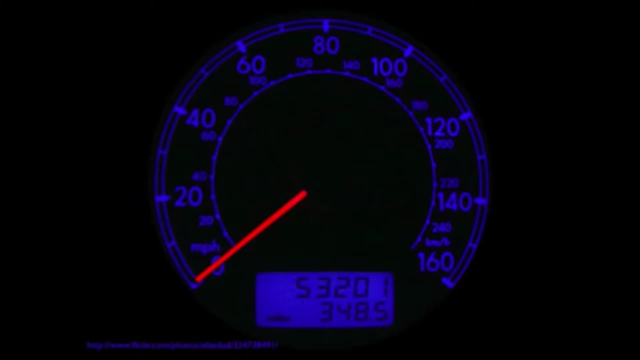 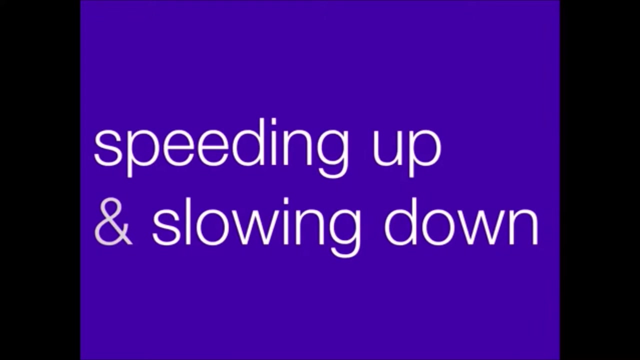 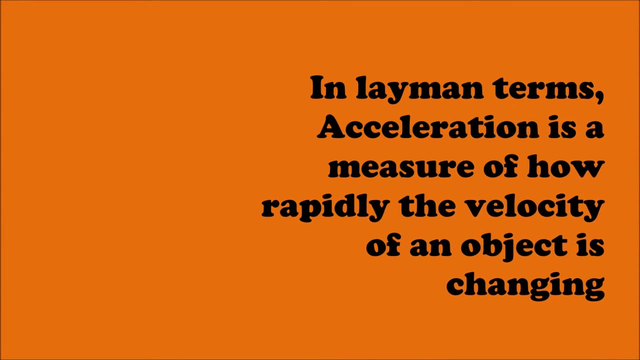 point 0 to 60 in 3.3 seconds. It's going from this to this. Acceleration is speeding up and slowing down. In layman terms, acceleration is a measure of how rapidly the velocity of an object is changing. It can be calculated by differentiating velocity. 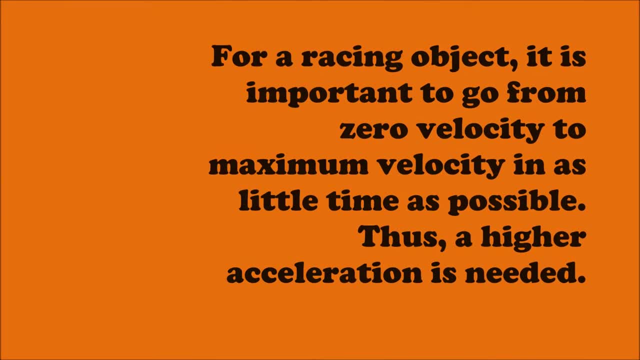 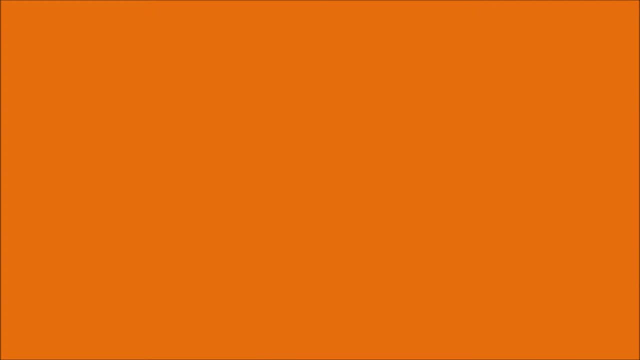 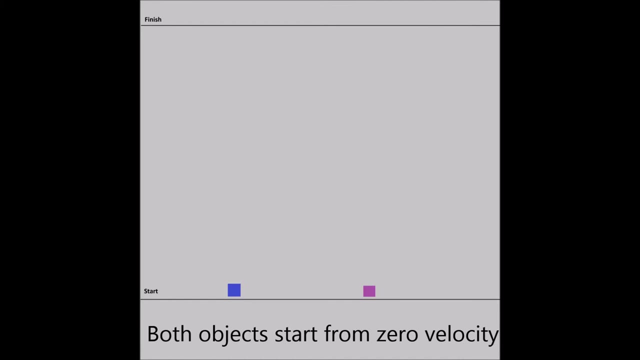 For a racing object, it is important to go from zero velocity to maximum velocity in as little time as possible. Thus a higher acceleration is needed. Both objects start from zero velocity. Blue has a higher acceleration, so it gains maximum speed sooner than purple and wins. 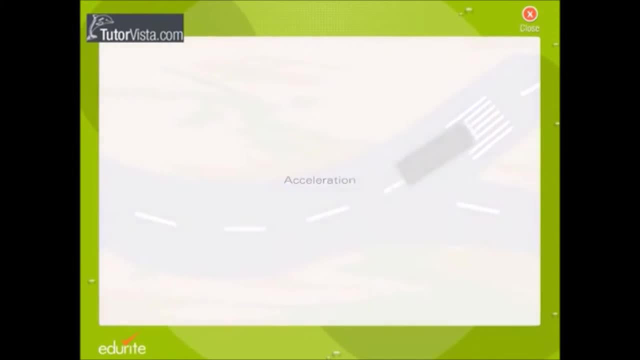 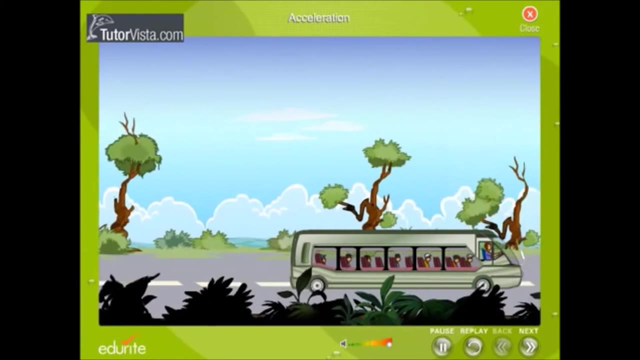 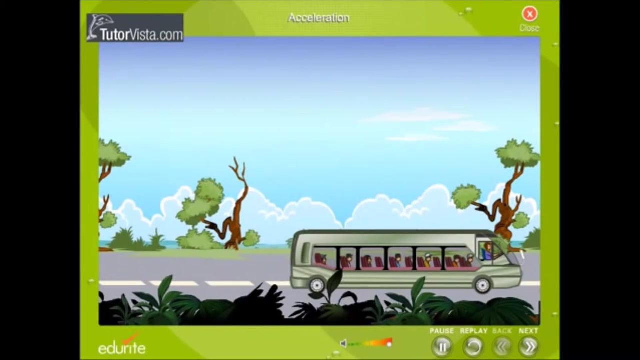 Acceleration? Did you hear the sound? What made the bus move fast? Why did the passengers jerk? Why did the bus screech? What do you think the driver did? All this happened because the driver changed the speed of the bus. Let us look at this again. 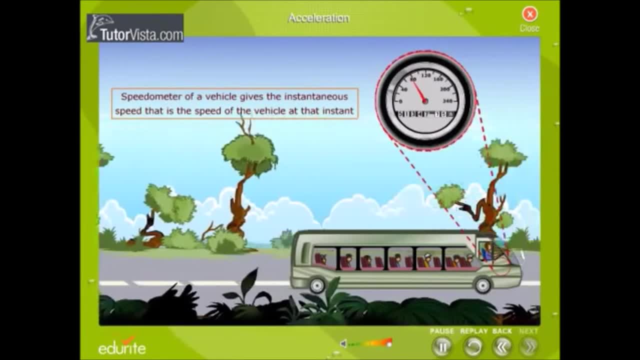 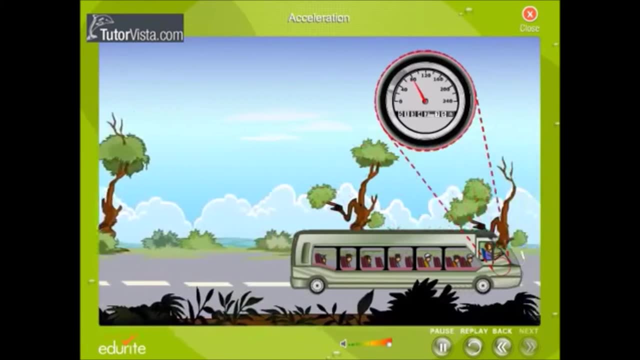 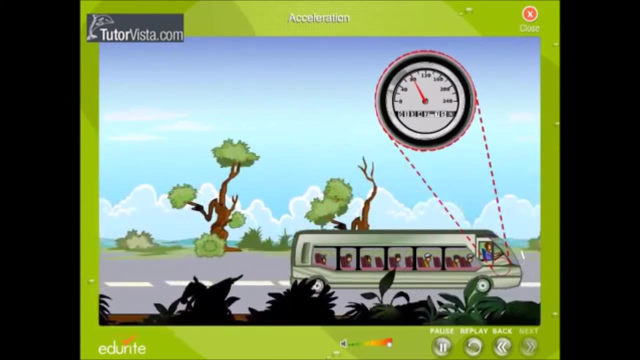 I'm sure you know that the speedometer of a vehicle gives the instantaneous speed, that is, the speed of the vehicle at that instant. Observe the movement of the needle of the speedometer as the bus is moving. We observe that the needle is moving, indicating that the speed of the bus is varying. 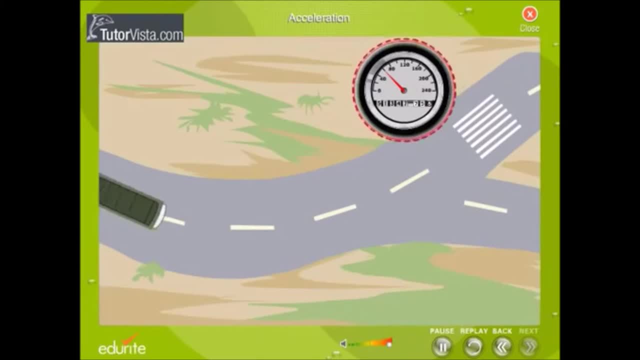 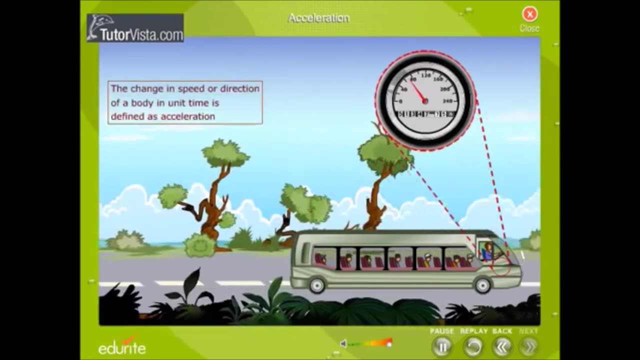 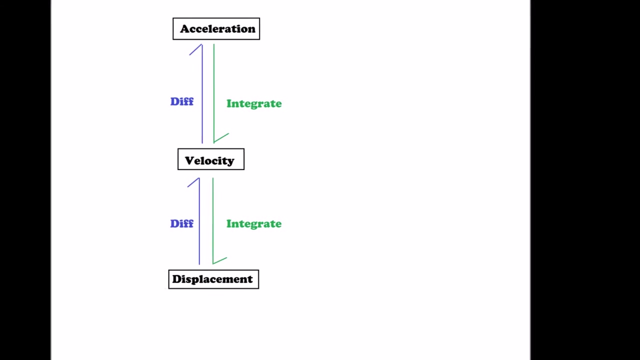 At times we observe that the speed is constant but the direction of motion of the bus changes. This change in speed or direction of a body in unit time is defined as acceleration. Differentiating displacement once results in velocity. Differentiating velocity results in acceleration. 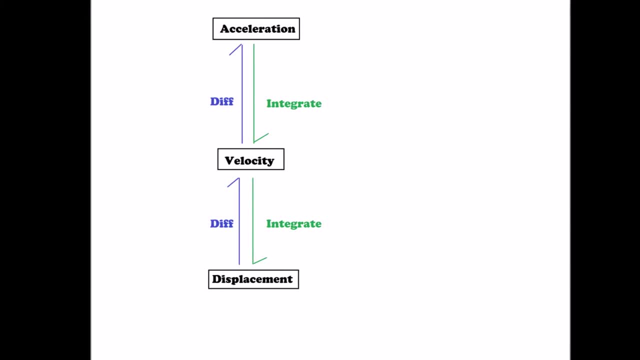 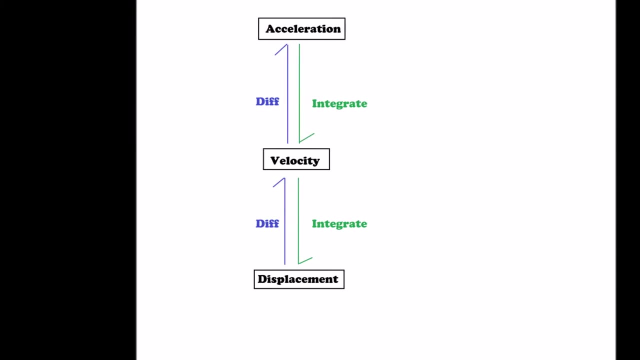 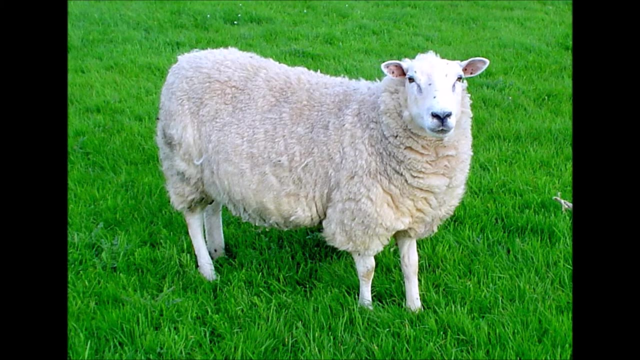 Integrating acceleration once results in acceleration. Acceleration once results in velocity. Integrating velocity results in displacement. The size of the population of lions and sheep in the jungle is related to each other, because a lion is a predator and feeds on sheep.